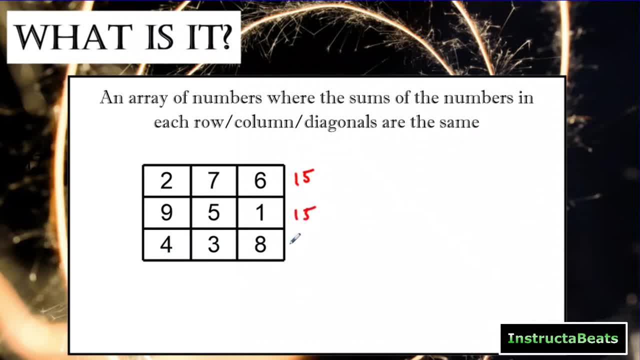 plus one, that's also 15.. If you add up four plus three plus eight, that is also 15.. If you add vertically: okay, if you add the columns two plus nine plus four would be 15.. Seven plus five plus three would be 15.. Six plus 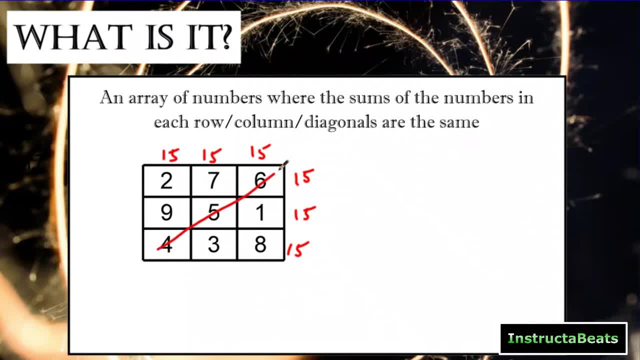 one plus eight would be 15.. And then also the two diagonals also equal 15 when you add them together. So that's why it is like magic. Another typical example of a magic square would be the five by five array. So obviously this isn't going to equal 15.. But if you add up each row, all five. 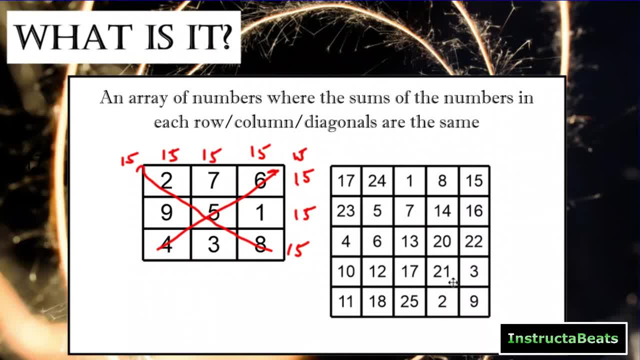 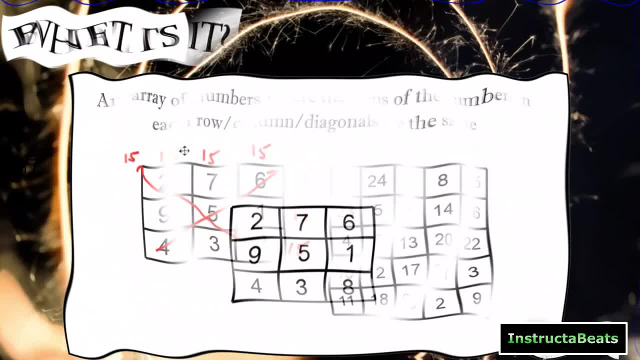 rows, all five columns and the two diagonals will give you the same sum when you add them up. So that's what a magic square is. That's why it is so magical. But what are the benefits of doing a magic square? Why, if you're a teacher, would you want to assign a magic square? Why, if you are a student? 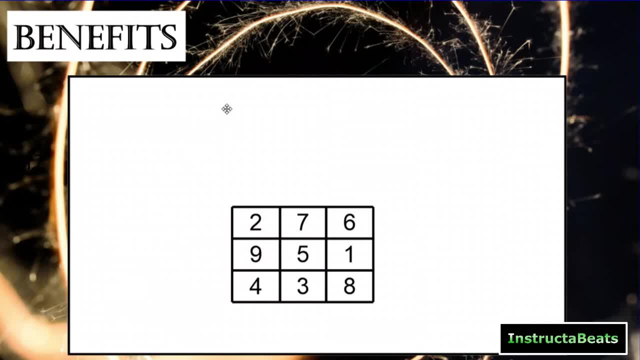 would you want to do a magic square? Or if you're just anybody, why would you want to do a magic square? So magic squares build mathematics. You can introduce and reinforce algebraic thinking as you work on these magic squares. It's a great. 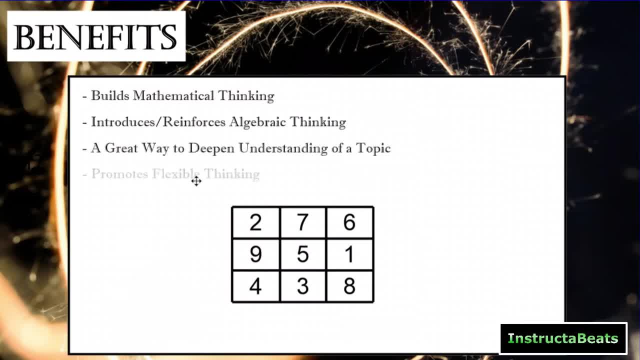 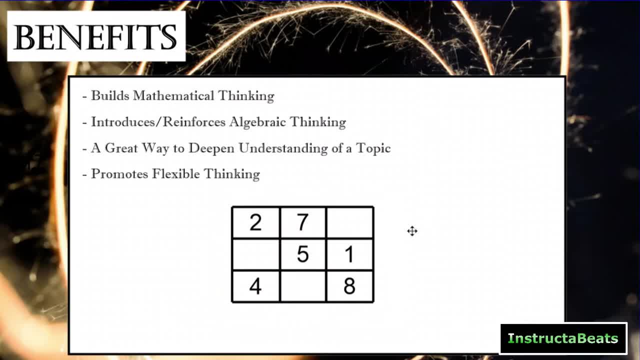 square right. You just have a couple pieces and now you have to find the rest of them right. So you're building mathematical thinking And you can increase the rigor of the thinking that you're doing by giving your students or solving a magic square with less and less numbers given to you right Now. 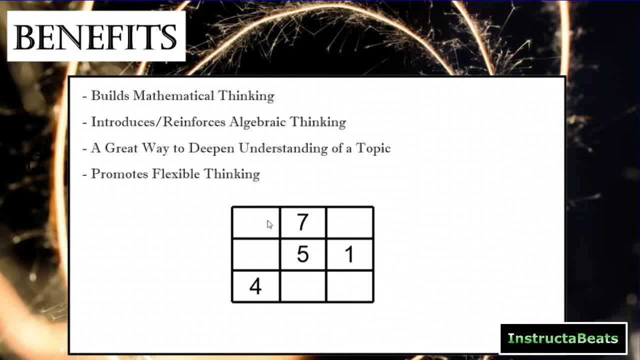 based on these numbers that I have given to you- even though I know I just showed you this- you would be able to figure out what these missing pieces are. And the great thing is, you can make these decimal numbers. you can make them fractions, right.